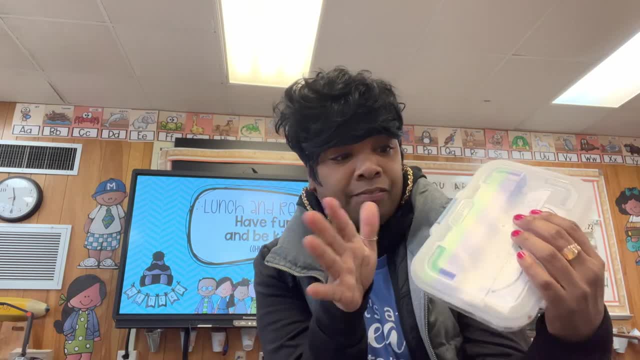 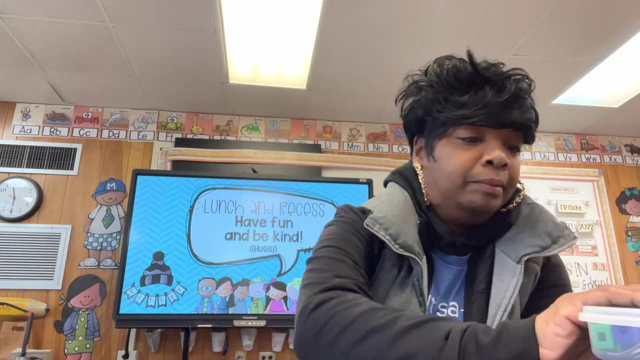 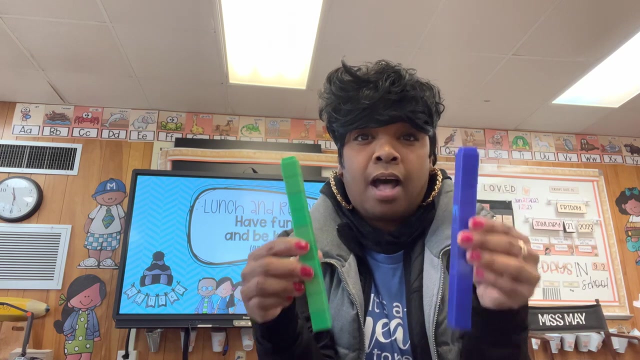 similar. I will put a link in the description box below if I can find some. But anyway, let's talk about what's in these bad boys. So every single student of mine has one of these and inside you will find two strips of tin from Unique Fixed Cubes. They have to be two different colors and 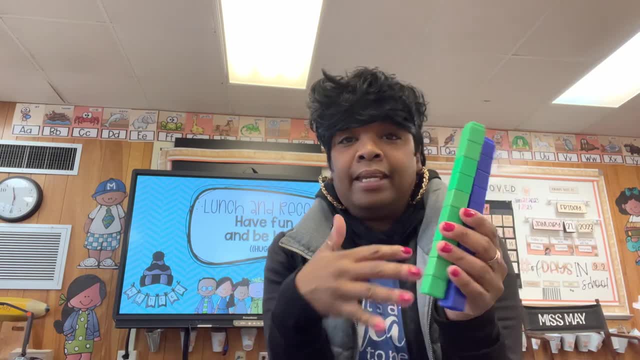 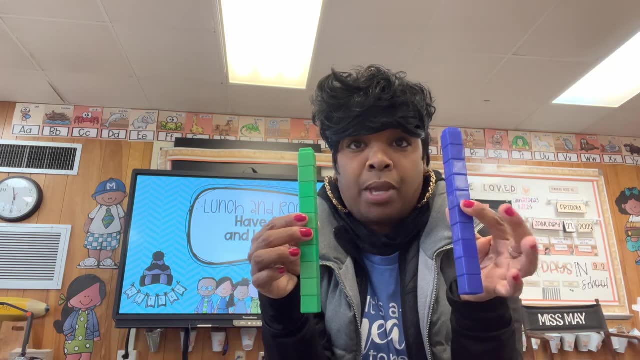 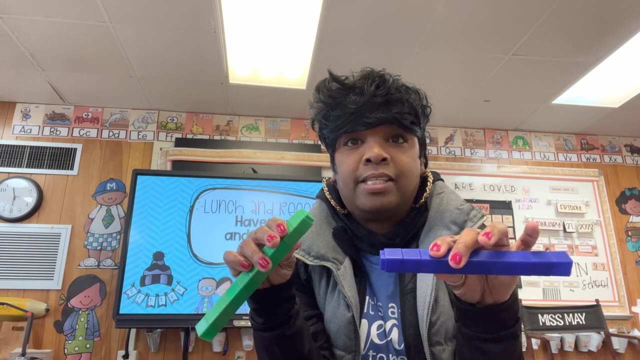 the reason being is because when we teach addition- adding, combining, joining, all that good jazz- we want the numbers to represent the different color. Okay, so if we were doing three plus two, they would take three cubes, two green cubes. join them together to find the sum, So we have two strips of 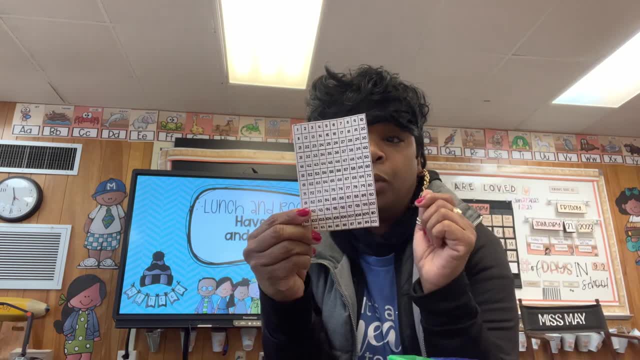 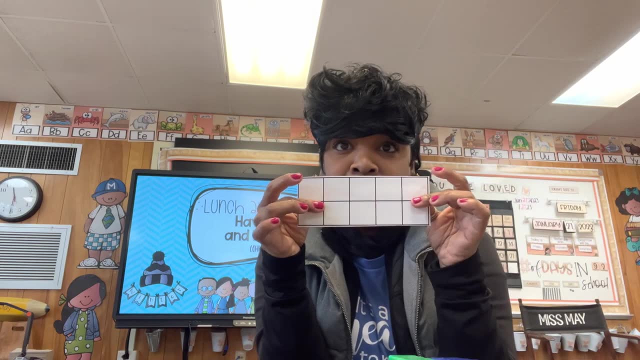 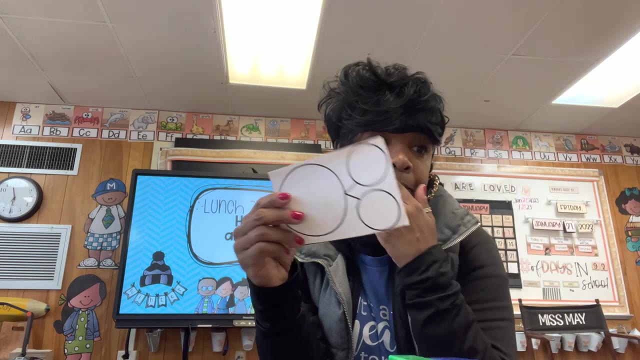 tin. inside We have a 120 chart, because in first grade 120 is the big number. Then we have a tin frame. Okay, the tin frame is a big popular frame in first grade. Then we have our number bond mat. They have a number. 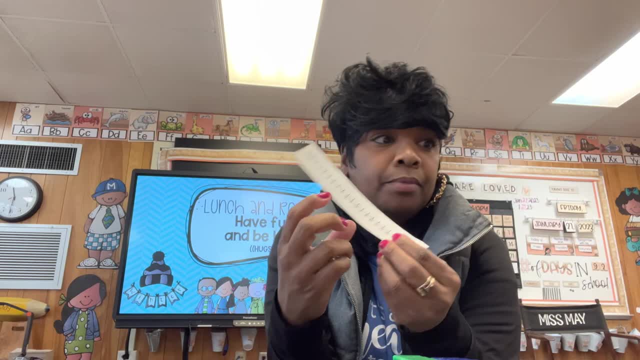 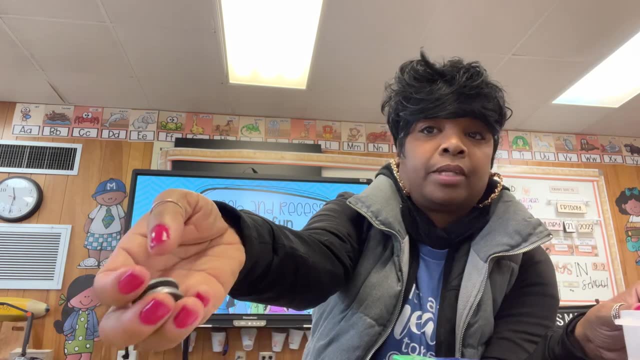 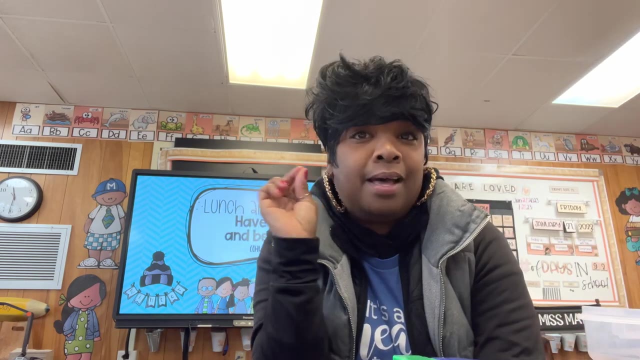 line 0 to 20.. They have some coins, because we just learned about coins, so they have some coins inside there. Okay, just little things, They change. and then they have a paper clip. Okay, the paper clip. we'll talk about why we have the. 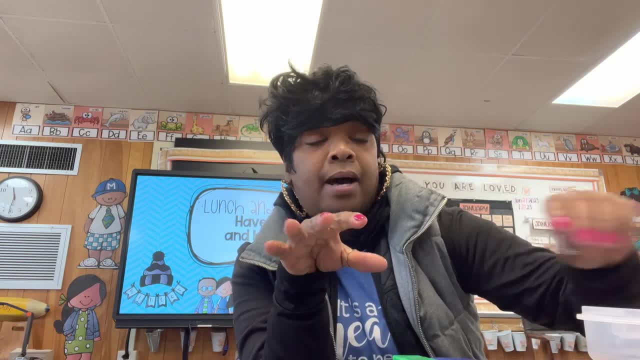 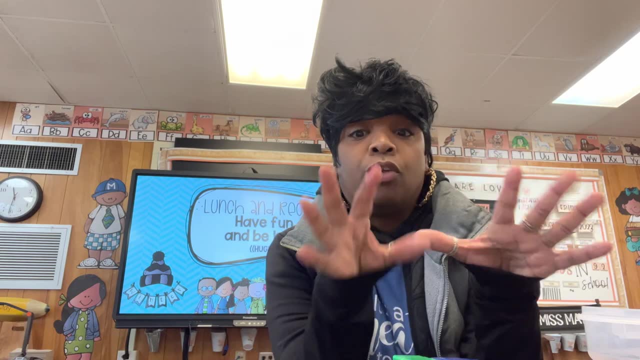 paper clip. So every kid has this inside their mass supply box Now, starting on day one at the beginning of the school year. they don't have all this stuff because I don't want them to be overwhelmed with all the materials. that that's inside their mass supply box. So what I like to 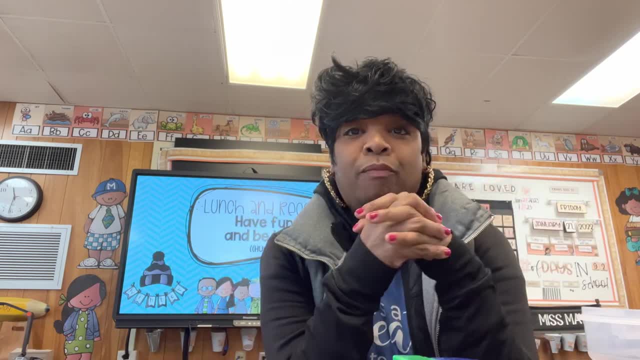 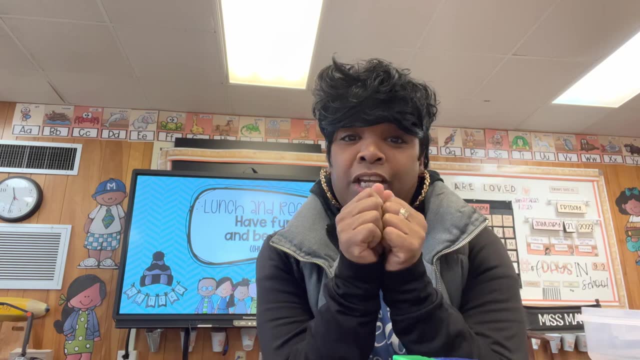 do is I like to model and teach them about the tool and how they can use that tool. Once I model, I have to do this. It's so easy to do. There's so many different ways to do it. There's so many different. 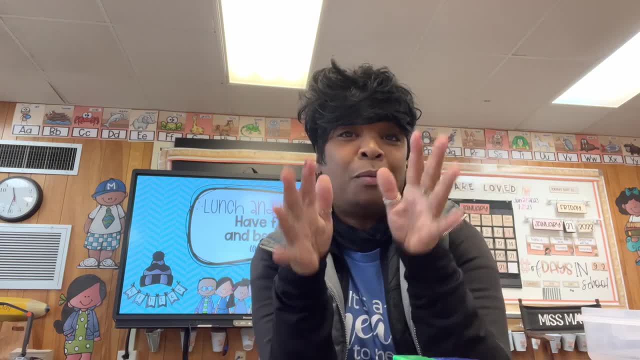 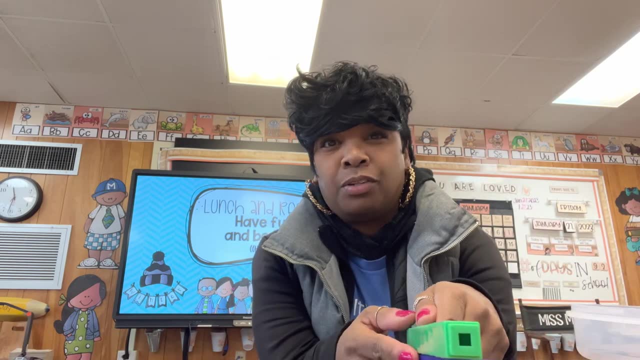 ways to do it. I'm a big fan of modeling. If you're an OG to the channel, you know how I feel about modeling to your students What things should look like, sound like all that good jazz. So model, model, model. So at the beginning of the year they just get this clear box and so, like the first, not 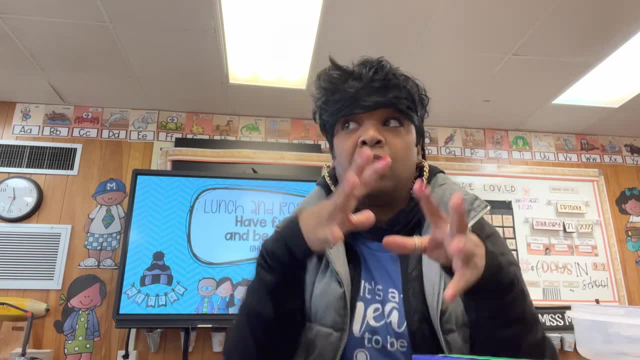 even the first, I'm lying. first day is always a blur, but probably about the third day of school I let the kids explore these snap cubes. I just put them all out on the tables. They explore, They build all that. Get the play out. 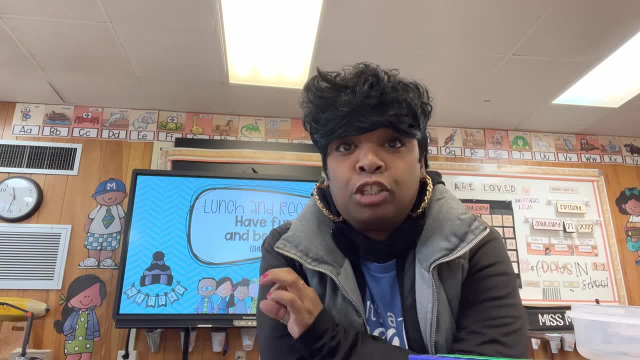 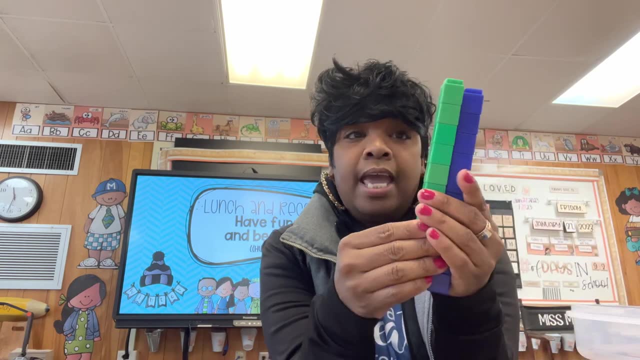 all that you want. And then I have them count their strips of 10.. They're responsible for counting their strips of 10.. I tell them they have to be two different colors And then I tell them that's what goes inside their mass supply box And that's the first thing that goes in there. 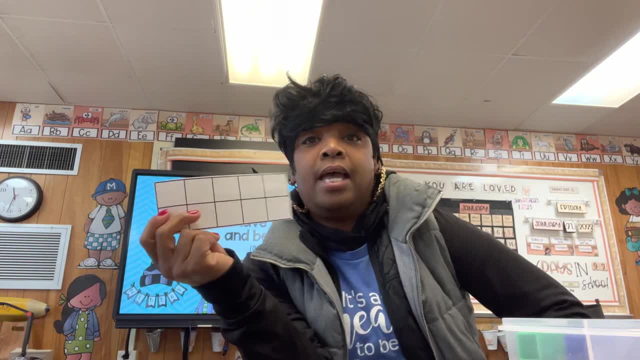 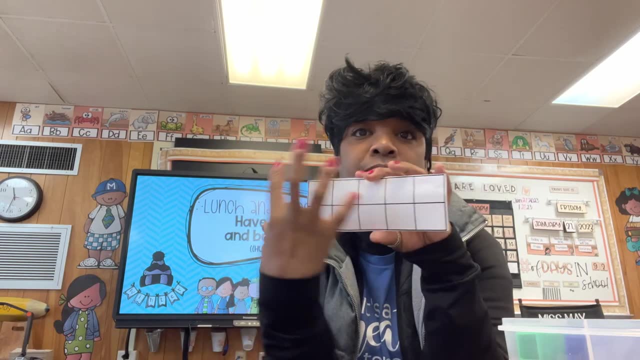 The second thing that I teach within that first week or two is about the 10 frame. We talk about the 10 frame a lot and we build on the 10 frame, We add on the 10 frame and all that good stuff Subtract on the 10 frame and then that goes inside their mass supply box so that they know. 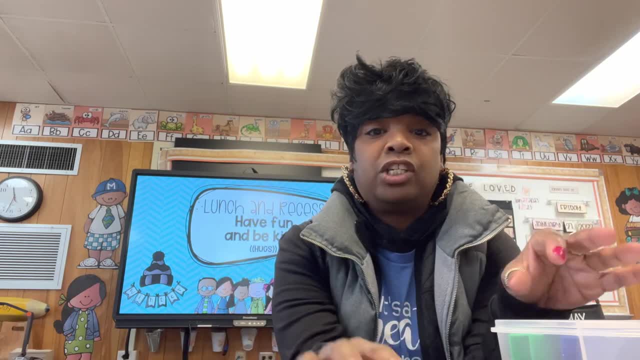 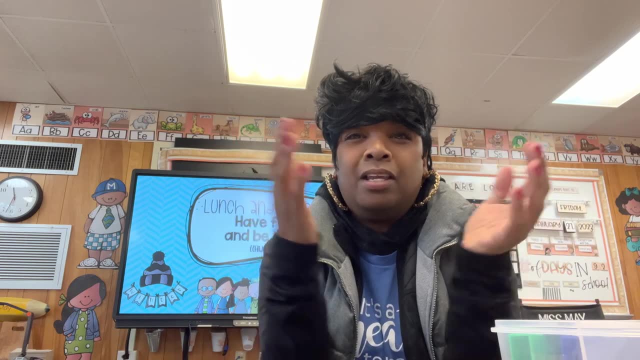 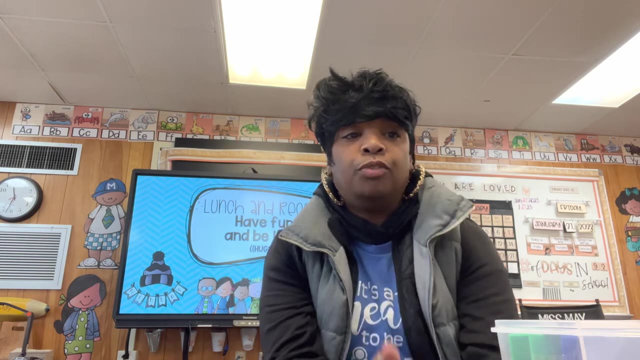 how to use those tools. So the key here is not to just give kind of like how I discussed many moons ago about anchor charts and putting everything all up at once. You know it's best to just gradually release things to these kids so that they get used to the tools that they're 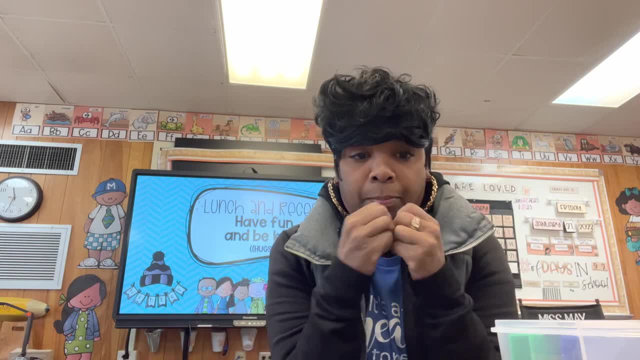 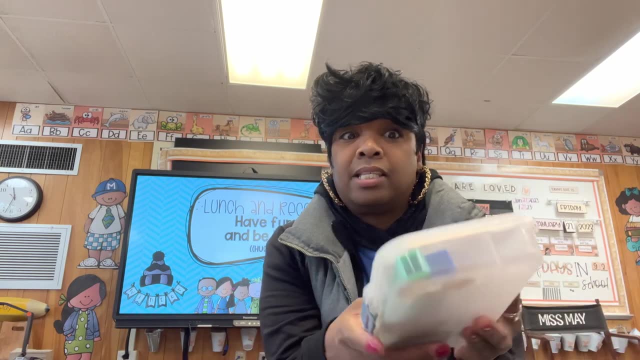 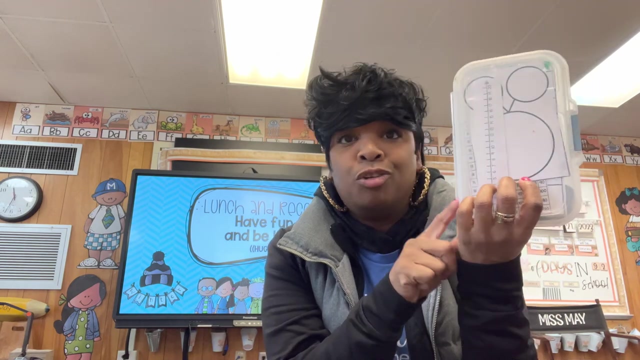 using and it's not just like a big blurb or a big blob to them. So we're on day 92. They have all this in here and the reason why is because that's been 92 days of lots of math. So they're very, very, very familiar with their box. They can use their mass. 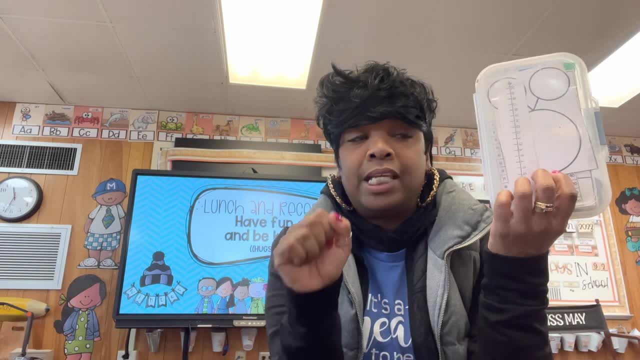 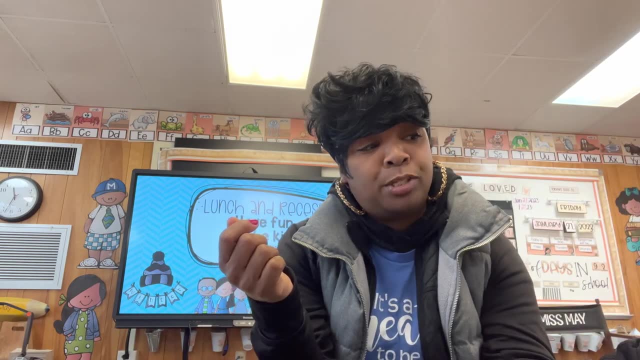 supply box whenever they need to, when they're working at their seats, when they're playing a math game. They don't have to take the whole box. They can just take whatever tool they like using and play their game. So love those. That's what's inside those mass supply boxes. 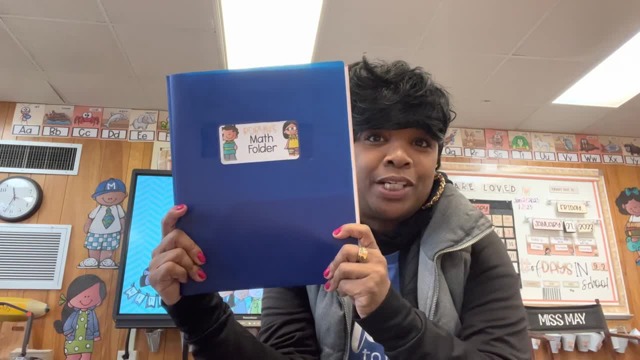 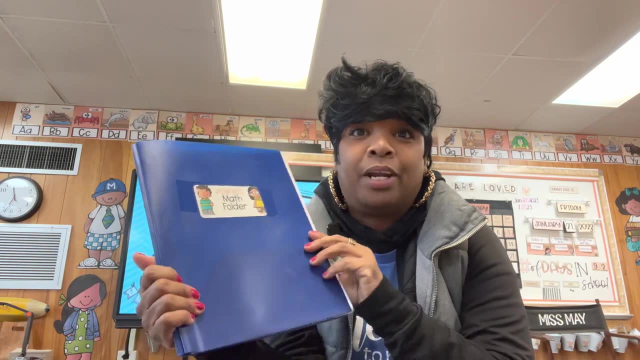 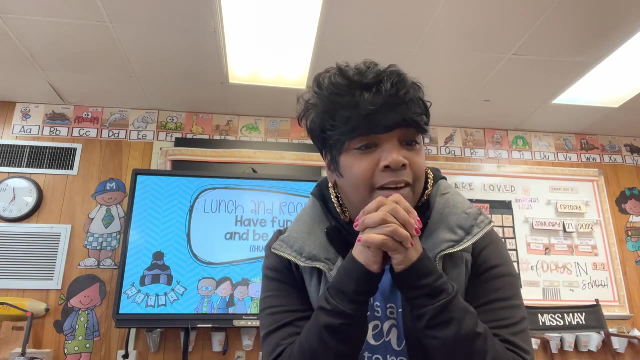 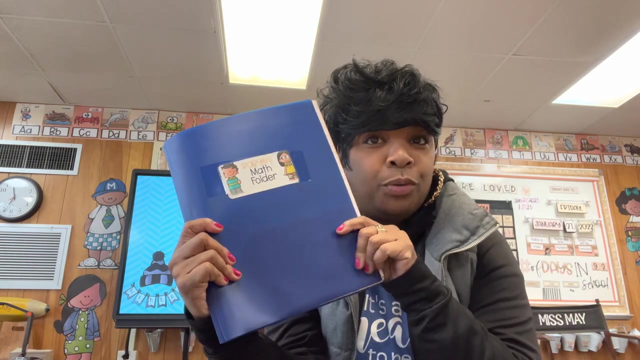 Next, the handy dandy math folders. Now my math folder consists of just math folder games. So during the time where we had to have blockers and masks and all that stuff, our kids could not share manipulatives and they couldn't play math games together. So math folder, math game folder happened. So they have a blue. 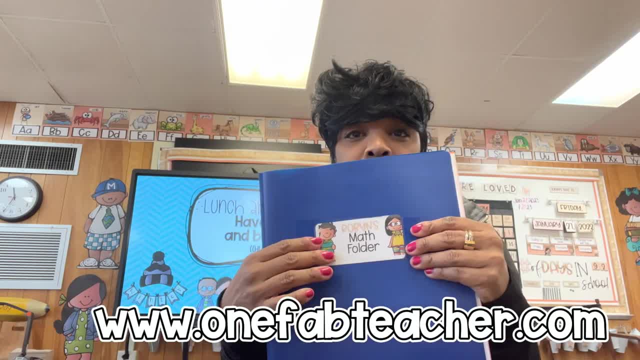 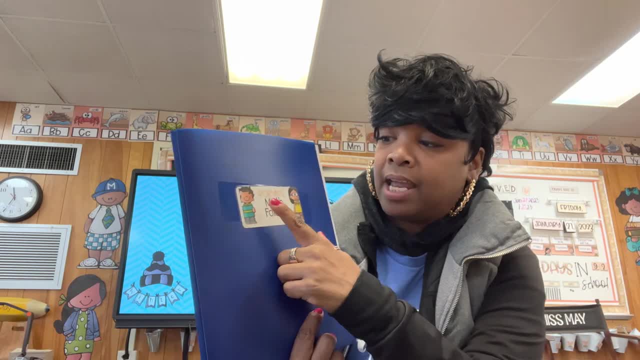 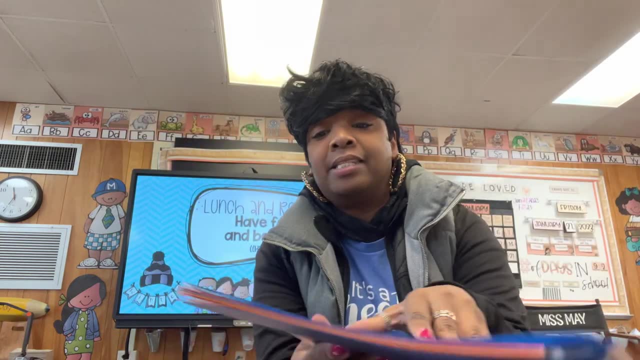 math folder, The label. you can find these labels on my website. I'll put a link in the description box for you. But basically I just put their name. It says math folder and then I put that packing tape to cover it And this lasts all year long. So inside the 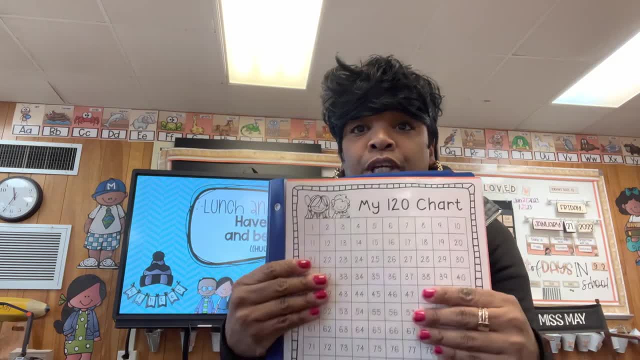 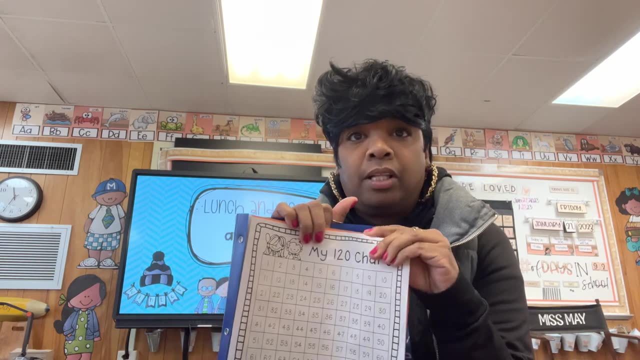 first thing that's inside. Now, at the beginning of the school year, when I'm getting these folders together before the kids arrive, I put inside about 12 sleeves, The clear protective sleeves. I put about 12 in there for them because they're going to be adding their math games in inside. 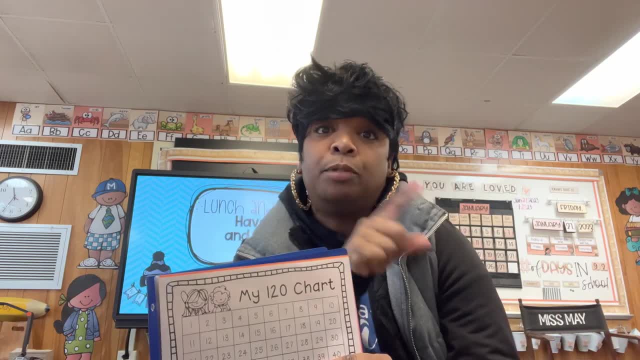 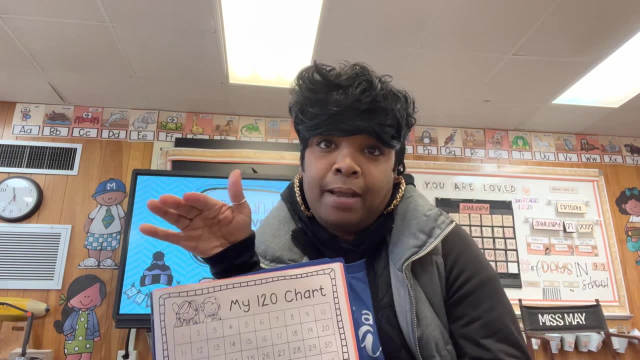 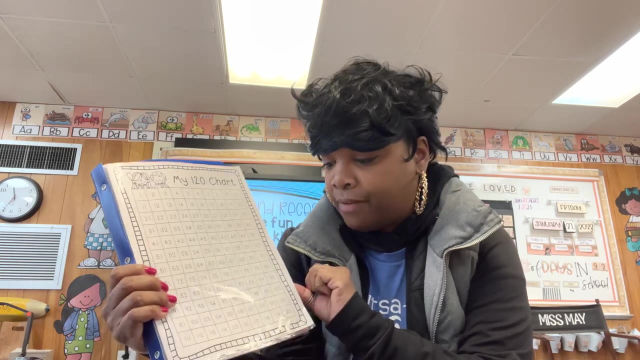 And it saves you a lot of time for doing, a lot of time from doing it for them. It's one thing to help them, But they also have their peers around them at their tables. that can help them as well. So, anywho, the first thing that's on in front of everyone's is the 120 chart. So we have our 120. 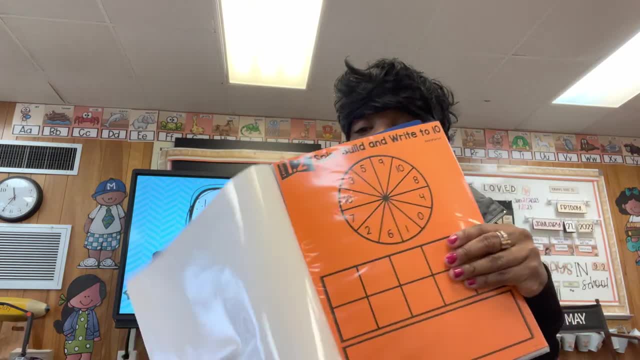 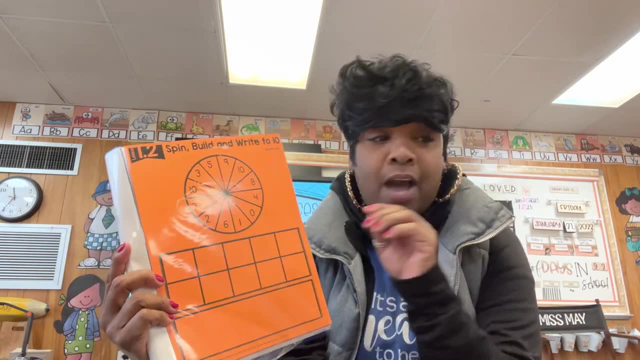 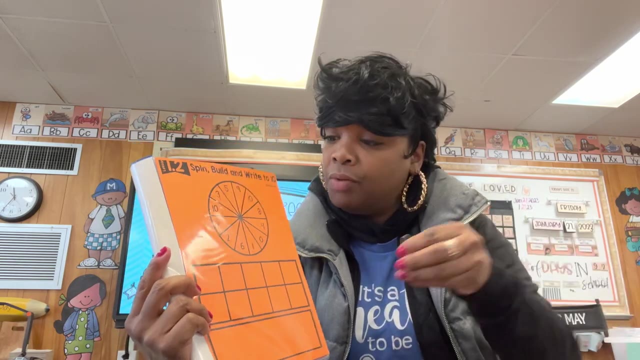 chart. That's the first thing in there, And then, when you open it up, we have the first game that I taught them, and it's called spin, build and write to 10.. Now that's where the paper it comes in handy, because the kids get a paperclip And what they do is they put the 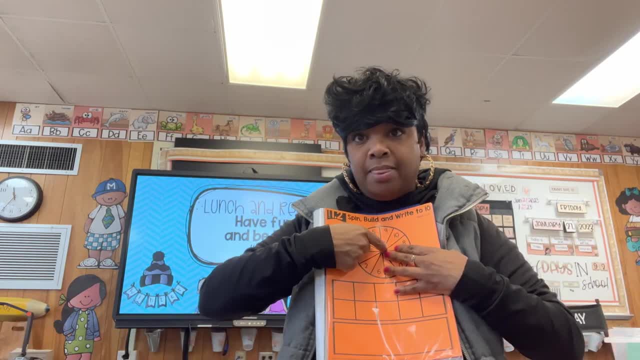 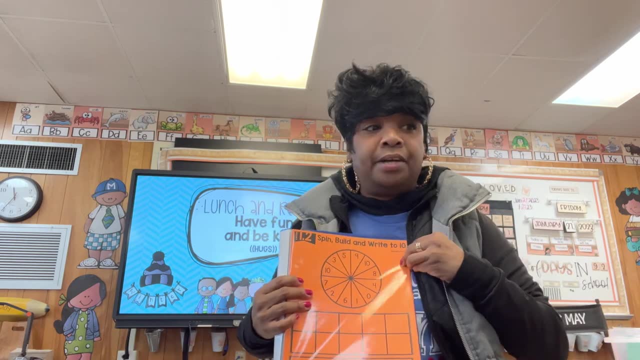 paperclip in the middle and the pencil. a pencil goes in the middle, So where my finger is right here, that's where you put a pencil and they just spit it and whatever they land on, they do what they need to do with it. Okay, So that's why they have a paperclip handy in their mass supply boxes. 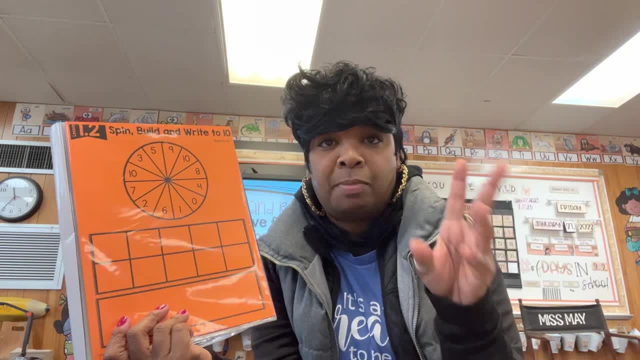 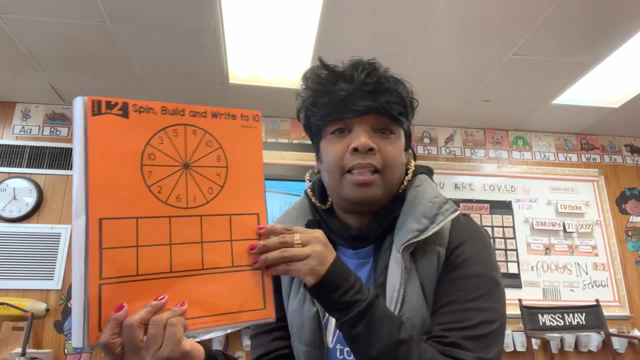 Do they lose the paperclip? Some majority of them are very responsible and can keep, but with it, now I've you, you will have some kids that just they, they lose it. They lose it. Like I gave everybody one or two and it's. you know, I get it. but three and four, Okay, We have 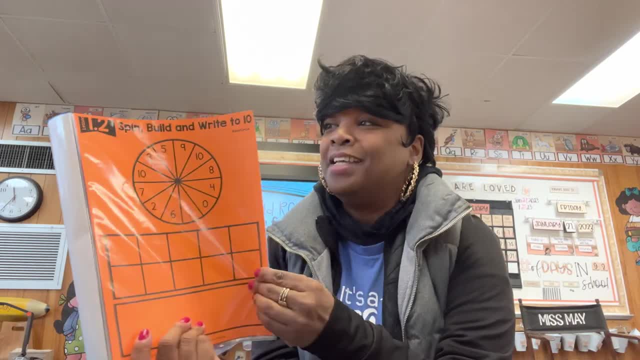 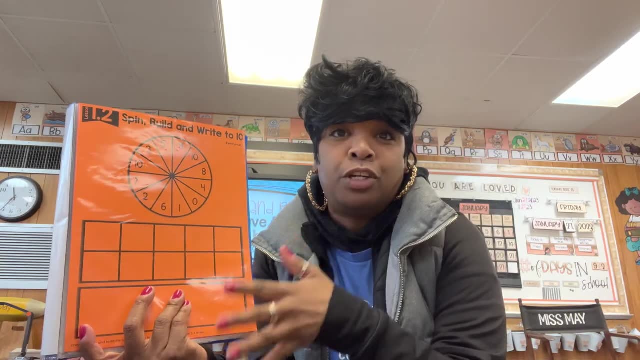 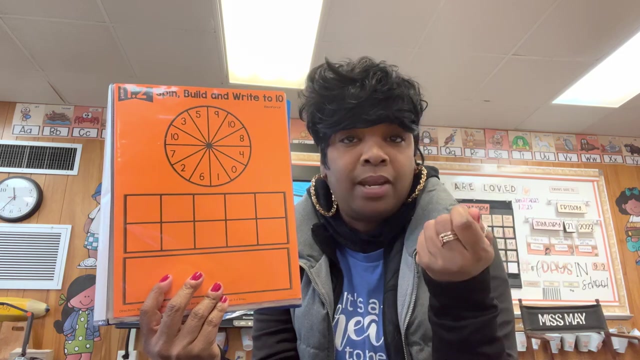 a problem You're, you're not being very responsible with your materials. So, anyway, so I give, I teach. I always model, model and teach the game to them, first so that they know how to play it, And once I model it to them, they all, I pass it all out to each, every, each and every one of them. And 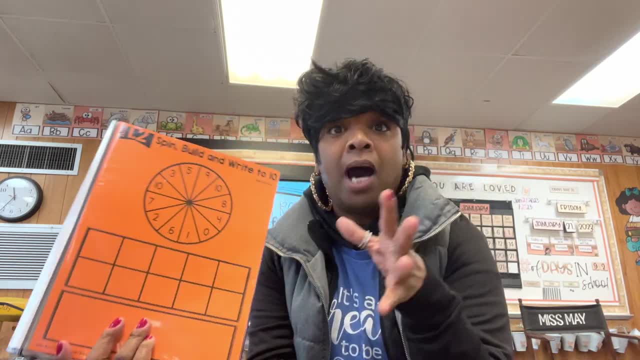 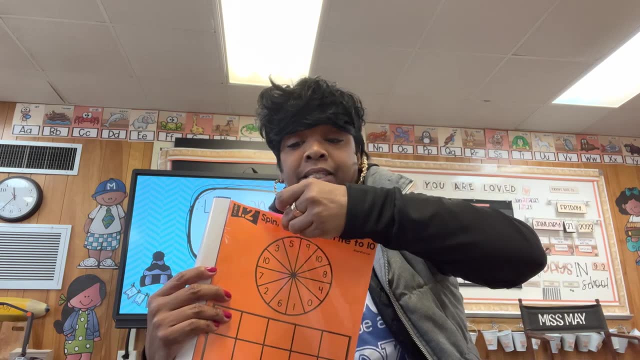 they put it inside that first sleeve And then I just kind of model how you put it inside the sleeve. So I have my own personal folder that I have and I model for them. Okay, Boys and girls, this is how you put this inside. 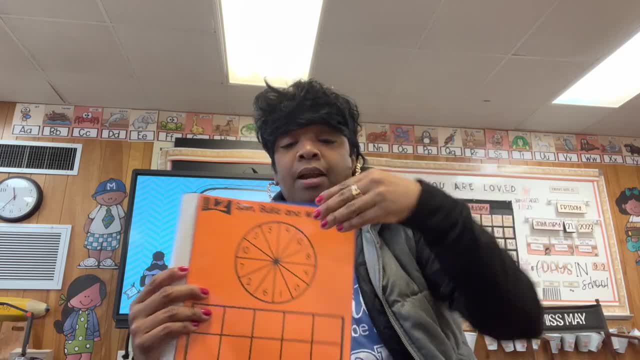 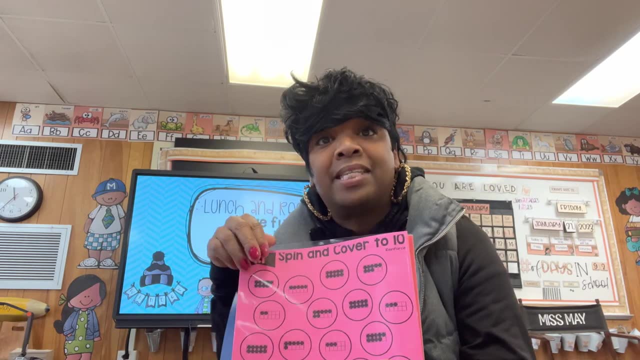 this math game inside your sleeve and they put it in there, And then when I introduce another one, they just add that game to the back of it in the same sleeve. So there's two games in a sleeve. Now I don't do front to back printing because I want to teach the game first before. 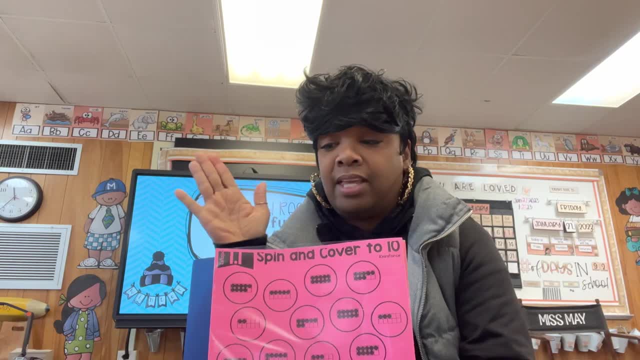 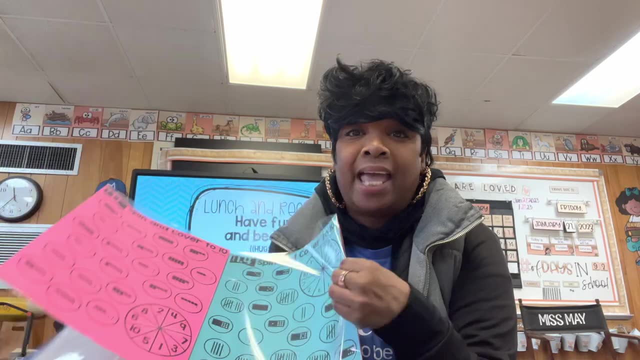 they put it inside here. It's just my thing, I just think that's important. So by the end of the year they just have all kinds of math games that they can play with play. I'll put a link in the description box below. 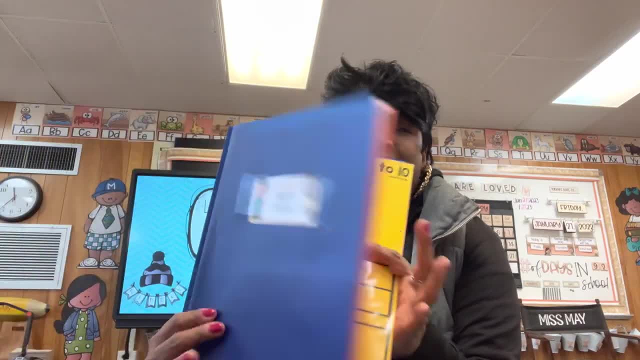 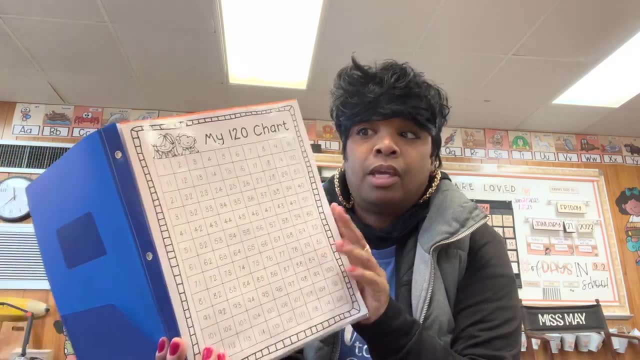 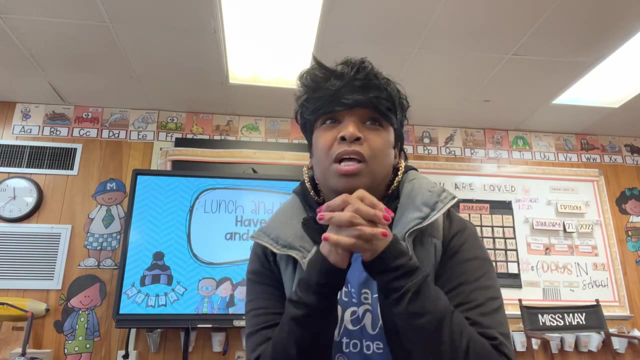 because I didn't make these. but these are amazing, but that's what's inside of here. It's just their one 20 chart and their math um, their math games. That's what they have in here And we just fill it up. And so these are amazing, because sometimes you don't, sometimes I just need 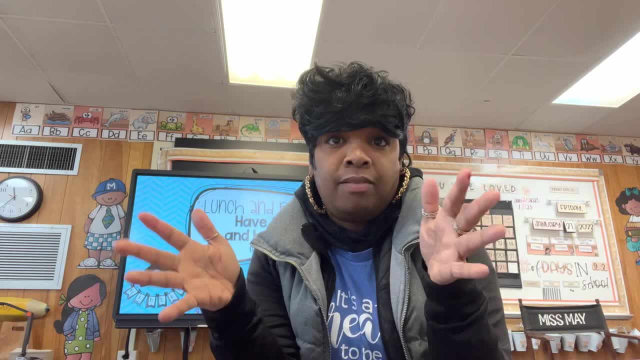 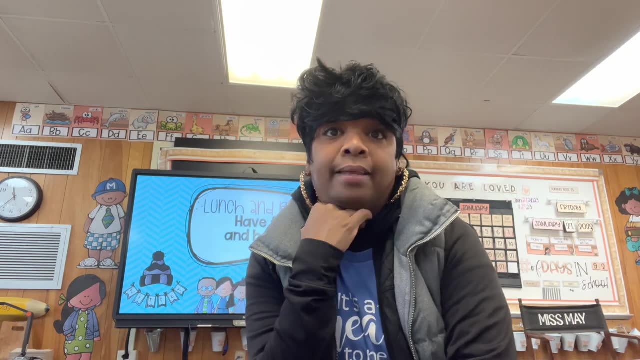 my kids to to do whatever assignment I give them. Once they put that in their finished folder, I'll say: I want you right now to get out your math game folder And I want you to work out of that simple. You don't have to get no paper, You don't have to. it's just not a lot, It's just simple. and 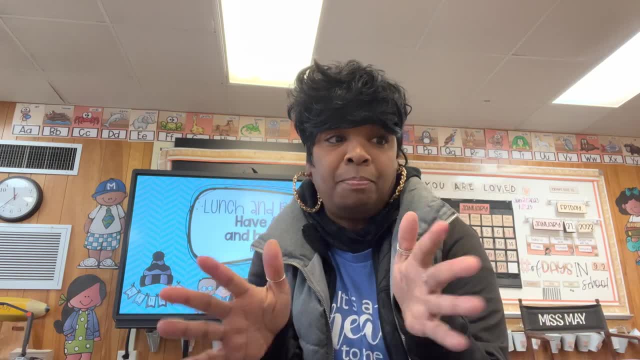 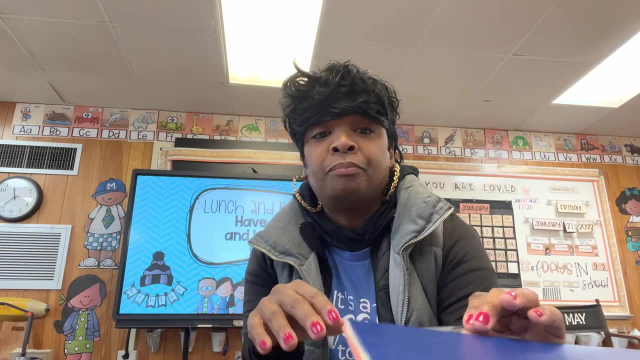 easy And, as teachers, especially this day and age, simple is what we need. We want to work smarter, not harder, And this is also great for a sub Like: if you're, you might have a true emergency where you're like: I have no clue where some 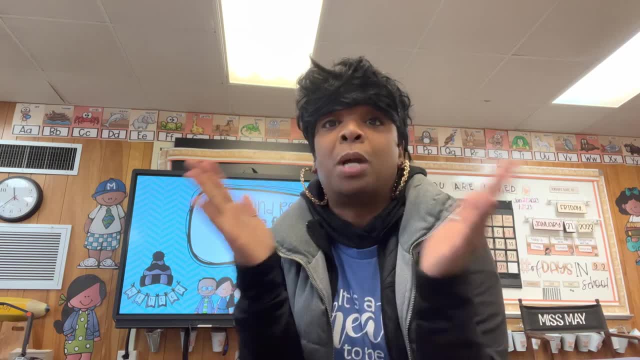 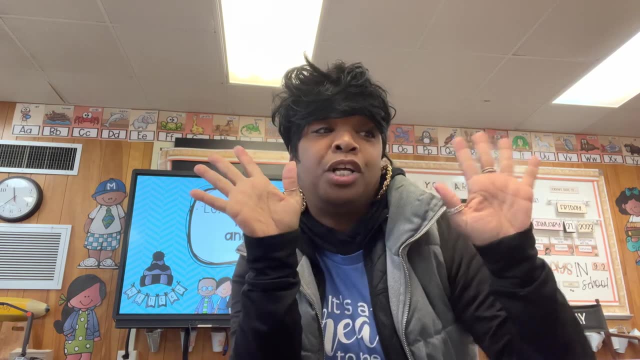 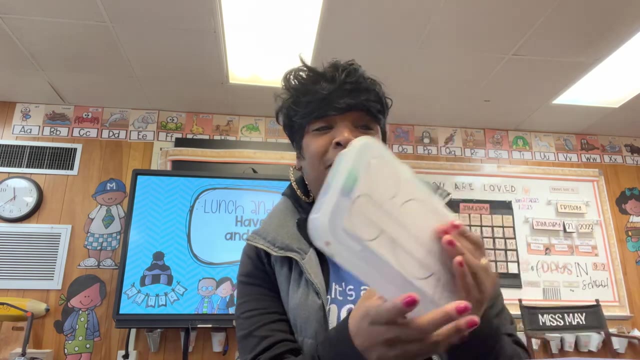 papers are to make copies. You just can't, I don't know, You just don't have stuff. This is perfect. Please have them play a math game out of their math game folder. Simple to the point. So I hope this helps you guys. I hope this answered your questions, but you guys were asking me and you 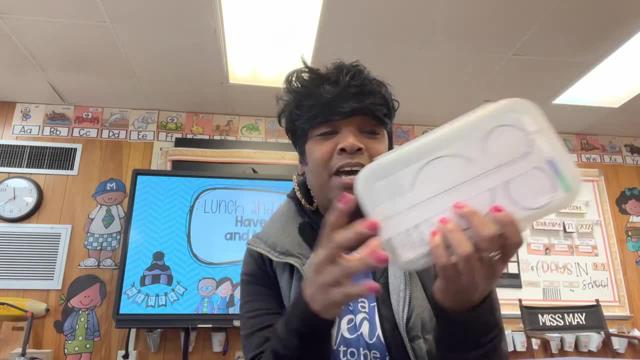 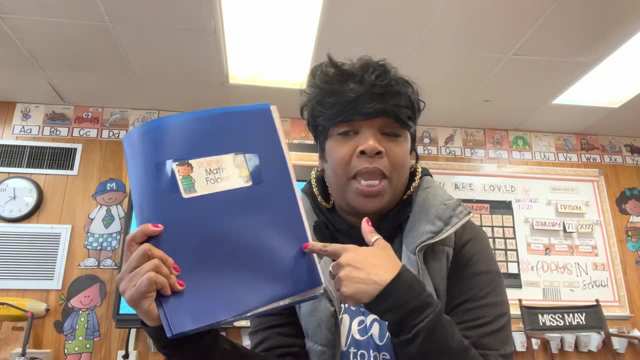 guys know I will do my best to show you, help you, tell you all that good jazz. So math supply boxes and math game folders. Okay, You can't beat it again. Like I said, these labels here. you can find these on my website. I'll put a link in the description box. 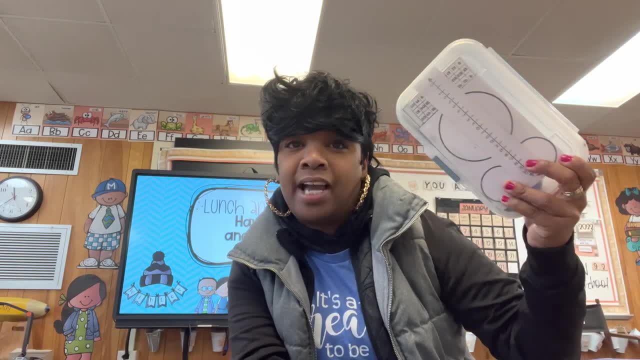 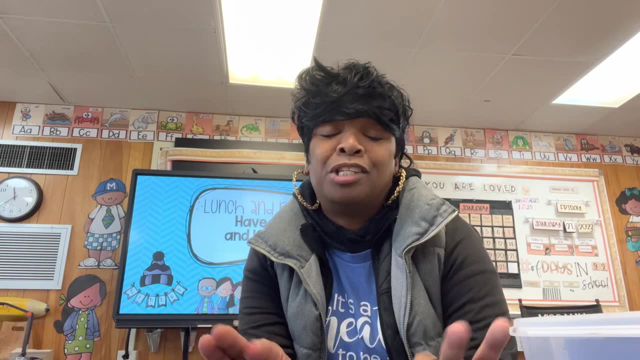 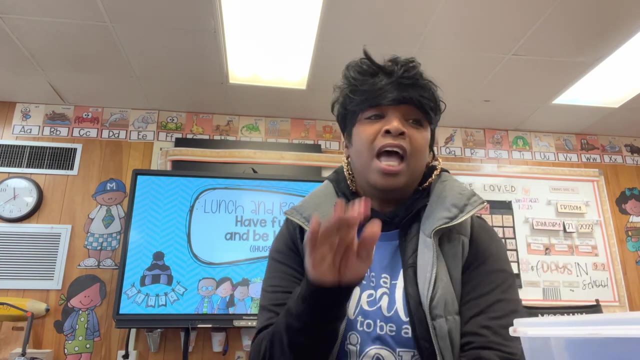 below and I'll try to see if I can find these or something similar, or y'all what I love about our comment section or people are just so like helpful and so kind And so, Oh, you can do this. Oh, I hope you do that And I love it. So if you have something like a math supply box, that